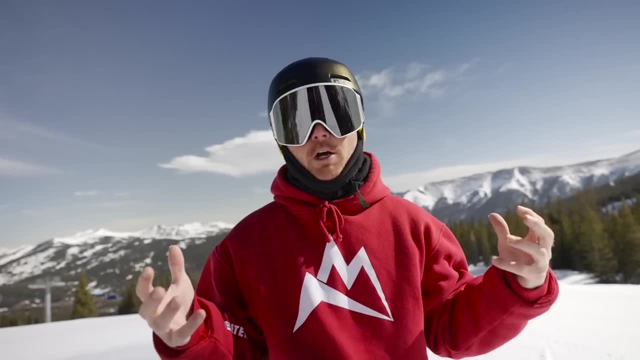 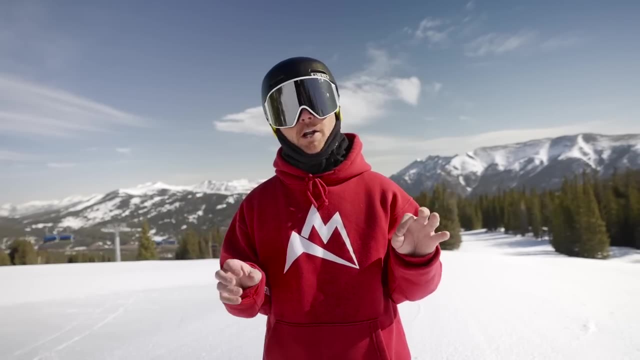 Just kidding, You're gonna go hit a ginormous jump. Well then you're also gonna need the ability to go fast, in a strong body position for going extremely fast. We got to understand what the fall line is If you had a bowling ball and you were roll it down the hill. 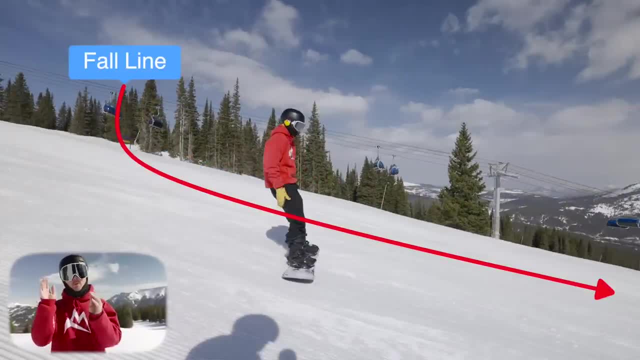 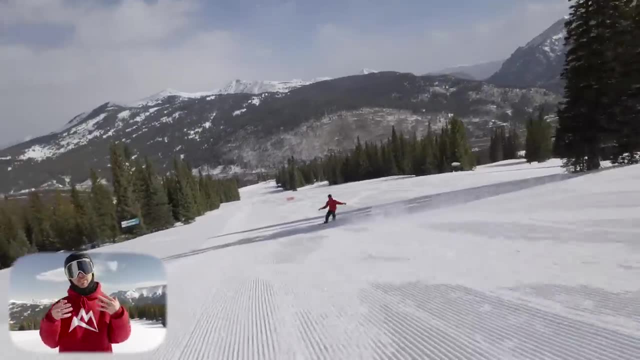 Where exactly would that path of the ball go? now, when we point our board down that fall line, We're gonna accumulate the most amount of speed as we turn our board across the fall line. That's when we slow down. any time you want to go fast, point your board down the fall line. 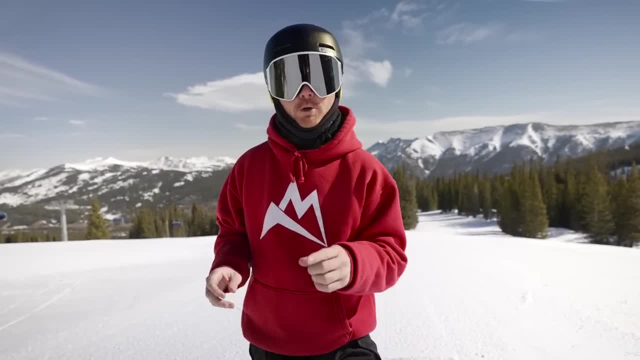 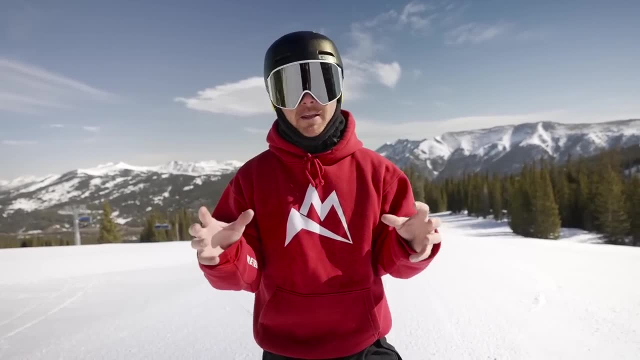 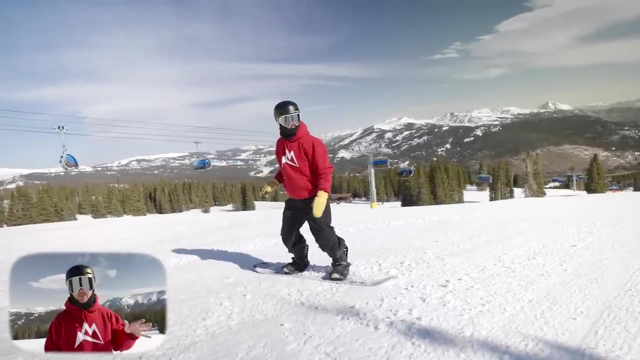 You want to slow down, Point your board sideways. pretty simple but very important to know. you got to have an extremely powerful, Strong stance that allows you to handle the terrain. first, You make sure your shoulders and hips are Perpendicular to the angle of your front foot. So for my front foot my binding is at 15 degrees. 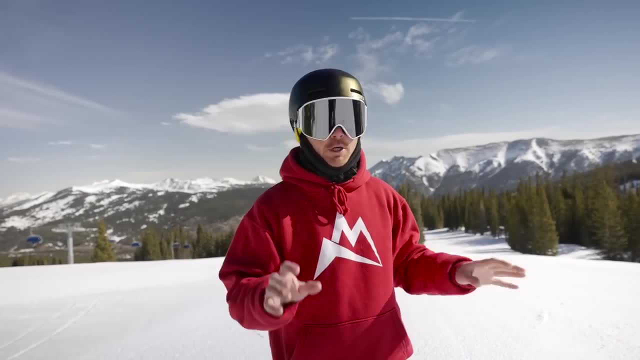 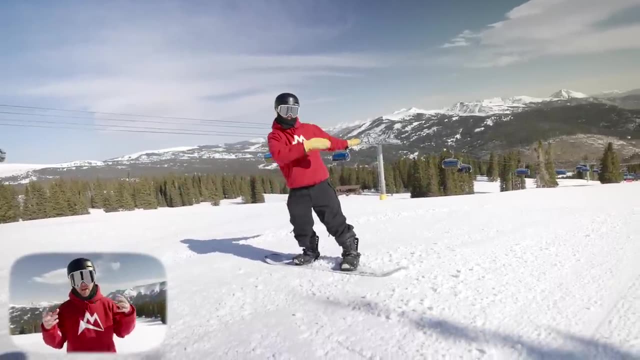 So I'll actually have my lead, shoulder and hips slightly rotated open, But you're gonna notice that I am not completely 45 or even 90 degrees open. I'm gonna be in a very optimal Position to allow me to have a greater range of motion, better performance and better balance. 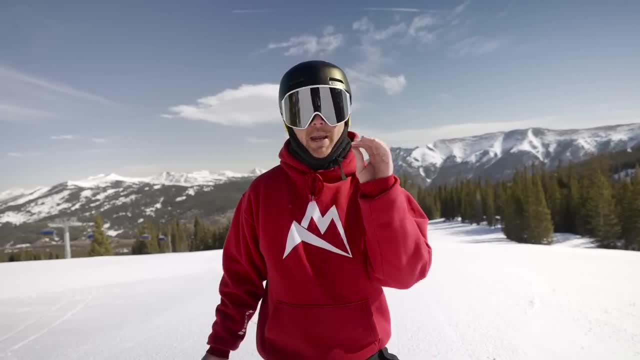 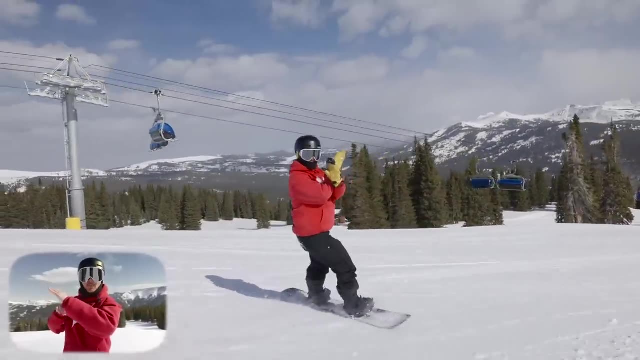 if your shoulders and your hips and your board Parallel to the angle of the Train or feature that you are on. So as you're going down a really gnarly slow, You want to make sure you have your weight distributed evenly between both feet as you're going down the mountain. 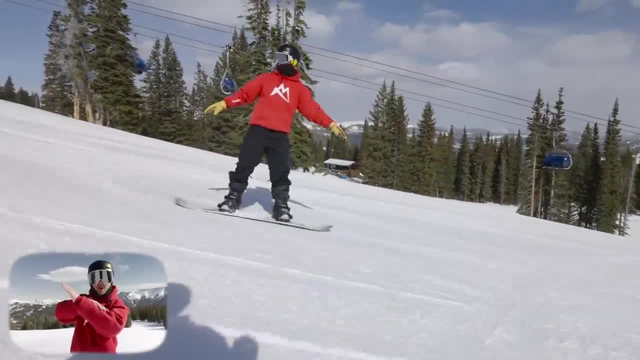 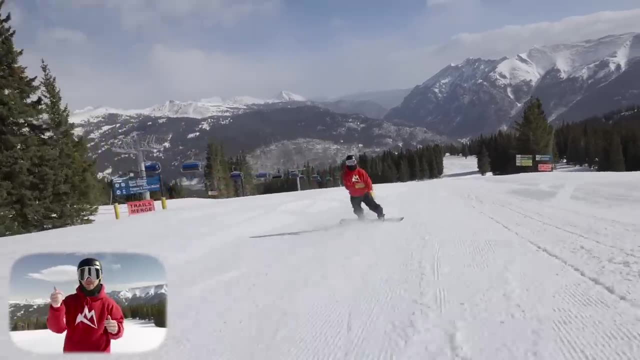 But if I'm not parallel, Essentially that means that all my weights in my back foot, my shoulders, are up and I'm not in a optimal position to be able to go fast and handle anything that's thrown at me. and the last big, fundamental aspect of a strong stance is keeping your weight over the 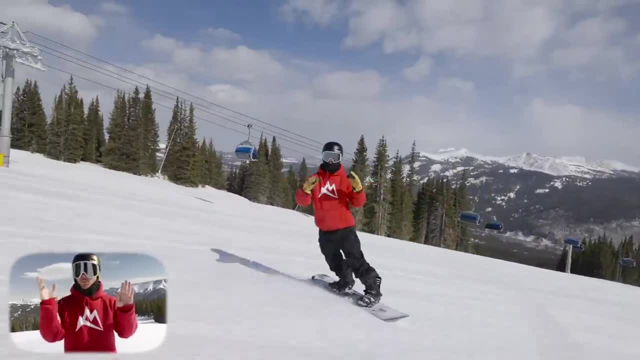 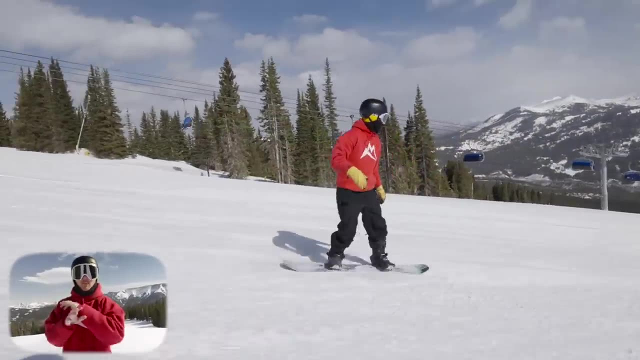 effective edge. so anytime my weight is on the wrong edge, I catch an edge and crash. so that's extremely important. with that out of the way, we're gonna go do a couple drills on how to be more awesome at going fast while staying in control, being comfortable and sending it. so today's video is actually sponsored by 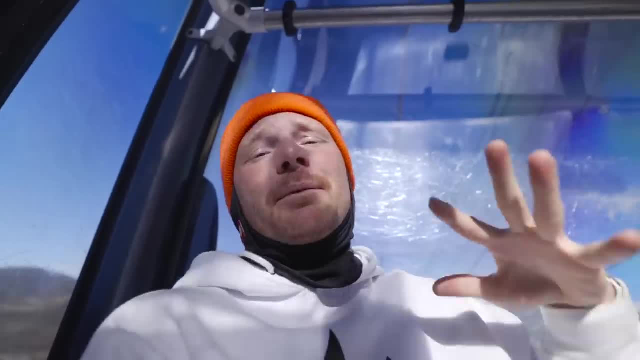 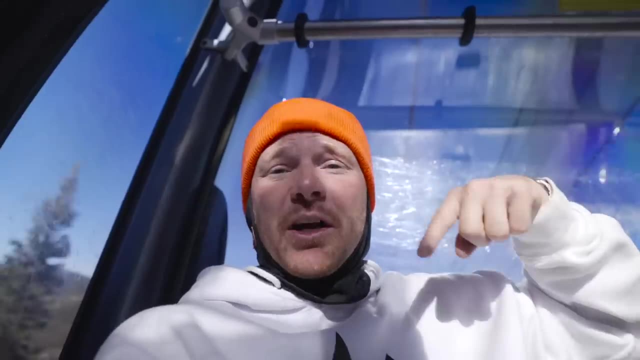 me and snowboardingsecretscom and in the membership, the ultimate goal is to make you as awesome as possible. so you're gonna get two mobility classes per week. you're gonna get coaching every week, where you jump on his live zoom call and you come vibe with me, and I'm gonna be offering two workout programs. 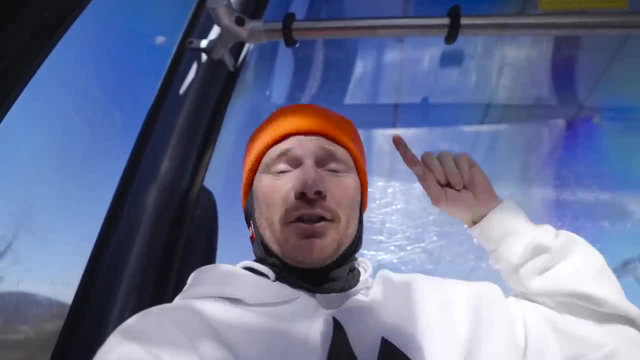 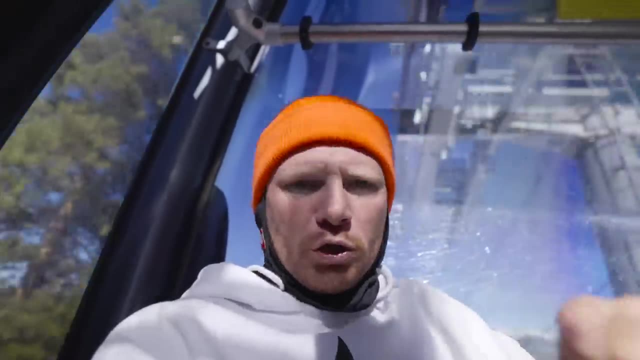 every single month. so sign up. the link is gonna be down below and you can sign up for seven days for free. try it out, come vibe with me and if you love it, hop on in. if you don't like it, all good. love you anyways, but try it with no risk. 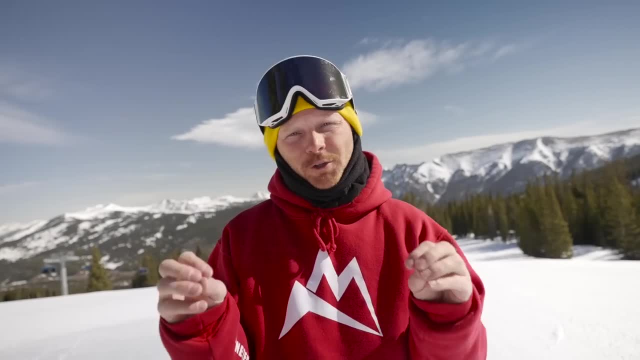 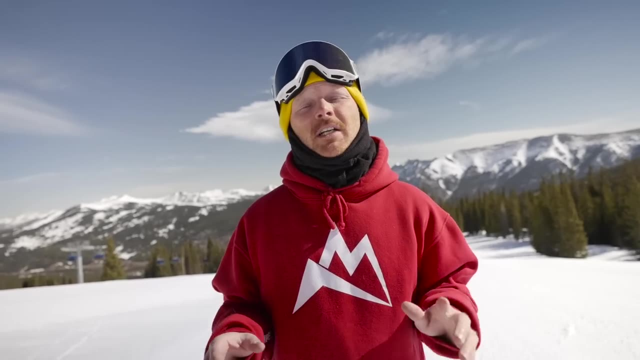 let's go. so now let's dive in to a couple useful drills. they're gonna change your snowboarding and make you way more comfortable, and you're gonna be able to do a lot of things that you're not used to when it comes to going fast. so the first thing that we're gonna do, we're gonna 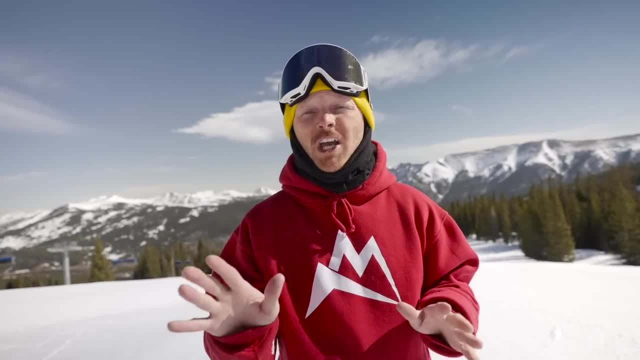 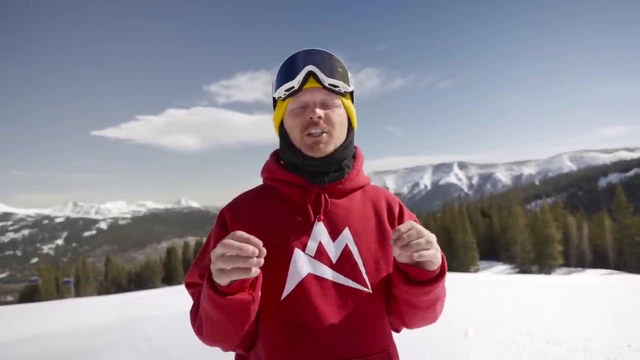 simply get comfortable pointing our board straight down the fall line on a flat base. so now you may not use a perfectly flat base all the time, but this is a great drill to understand. are you in the right body position now? the goal is to have our weight distributed evenly between our toes and our heels. 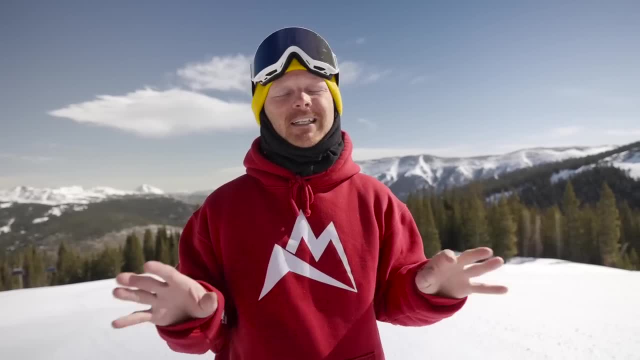 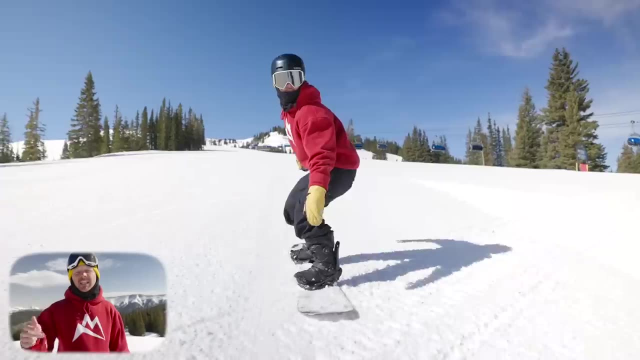 and our left foot and our right foot. whether you're regular goofy, it doesn't really matter. you're gonna point your board straight down the fall line and you're gonna count to three, one, one thousand, two, one thousand, three, one thousand, and then you're gonna stop. now, the goal is to 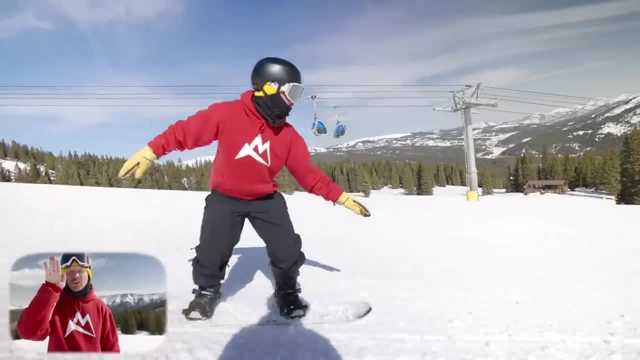 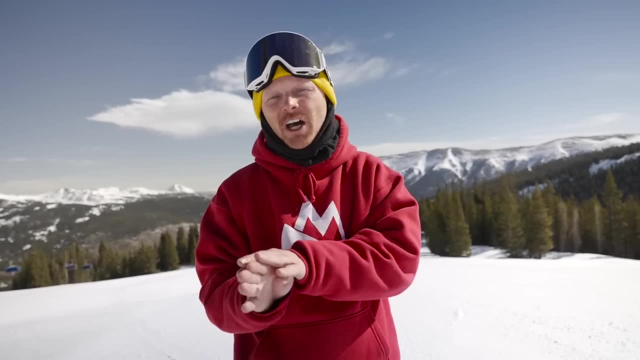 look back uphill in the path that you've created and to make sure that your board is perfectly flat. now, if you have a little bit more of a deeper carve on one side versus the other, that is an indication that you have your weight distributed wrong, in terms of being on your toes or your heels. so go ahead and 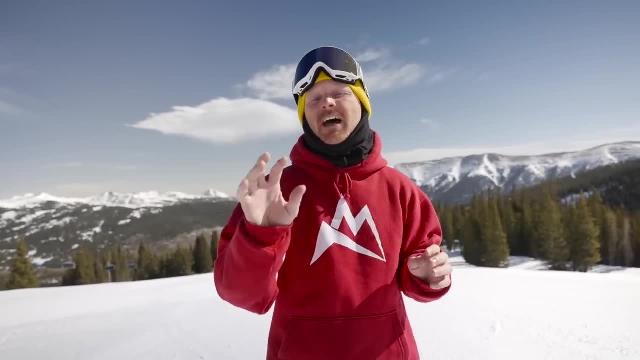 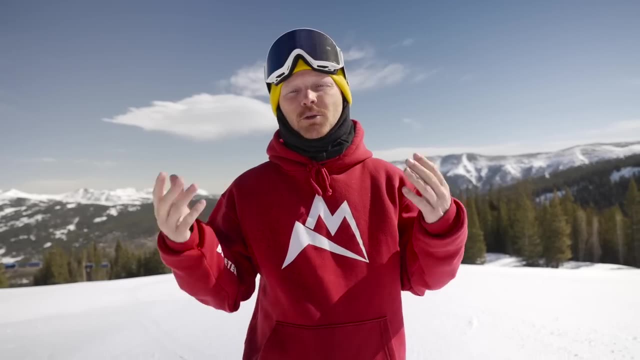 perform that task again, but really try to understand how to get my board to be flat. the other thing that you're trying to prevent is your board from rocking, and The other thing that you're trying to prevent is your board from rocking and rotating as you're doing this drill, if your board is going perfectly straight. 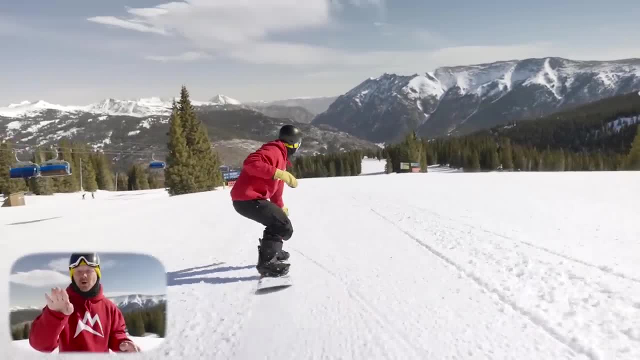 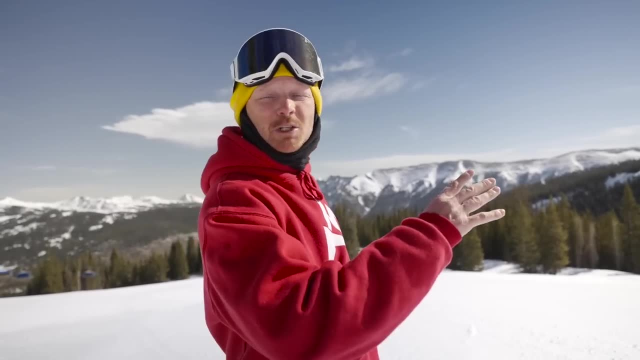 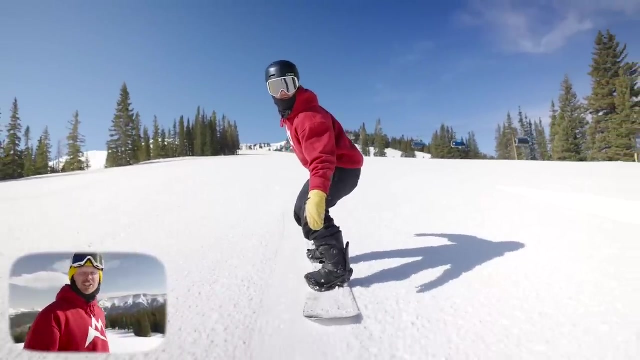 down the fall line. you're in a good stance. if the tail of your snowboard is trying to move sideways, even 45 degrees, that's an indication that your lead shoulder is way too open towards your heel side, causing the board to rotate. so the easiest way to correct it is get that shoulder back into that nice stance. 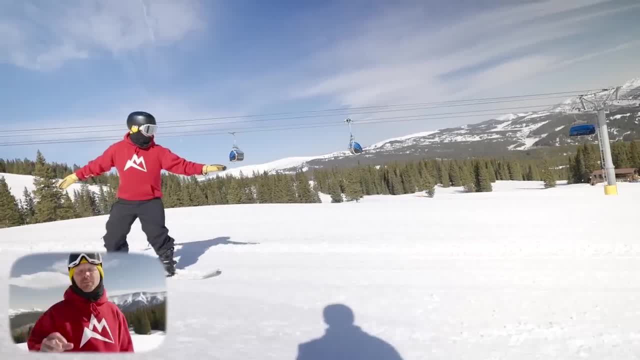 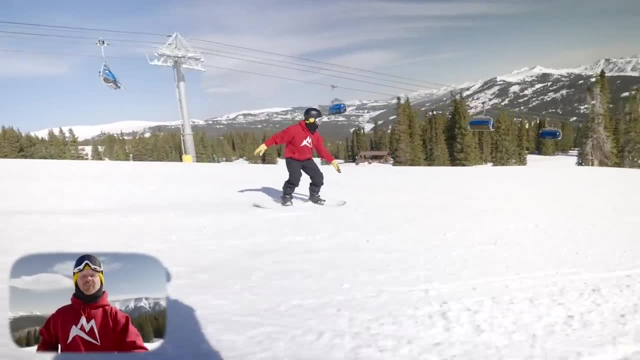 we talked about earlier. keep both knees bent and sink your belly button just a little bit. after you've done this drill, I want you to do it again, but let's make it a little bit more challenging by holding it for a five count. once you've done it for a five count, check the same. 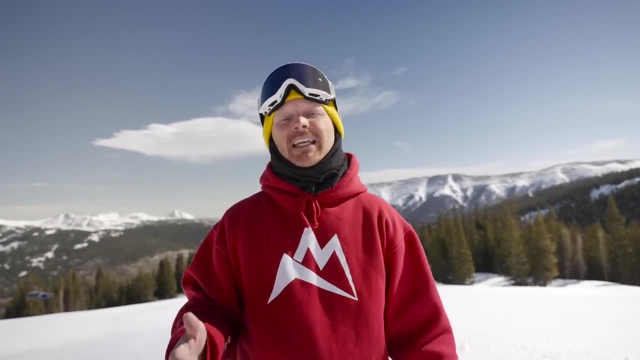 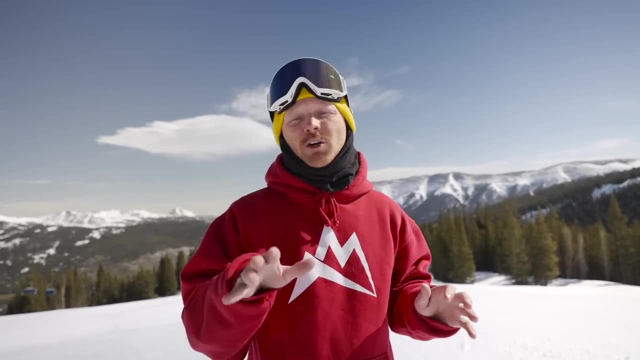 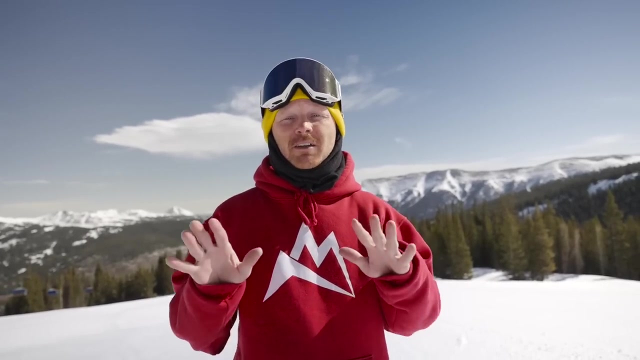 thing we just did on the three count, and then the next step would be add it to a seven count. can you hold a straight, flat base for a seven count without going to your toes, your heels or having your board go sideways? obviously, at this point you're gonna accumulate a lot of speed, so if you need to slow down, slow. 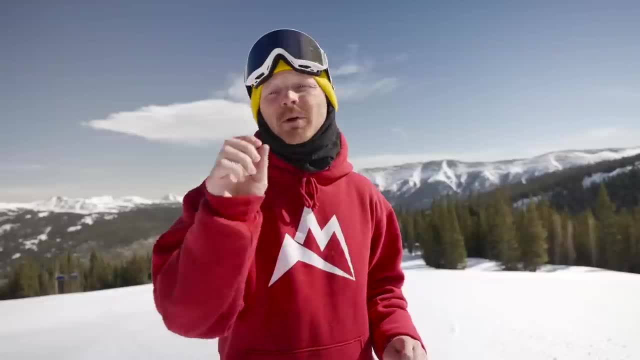 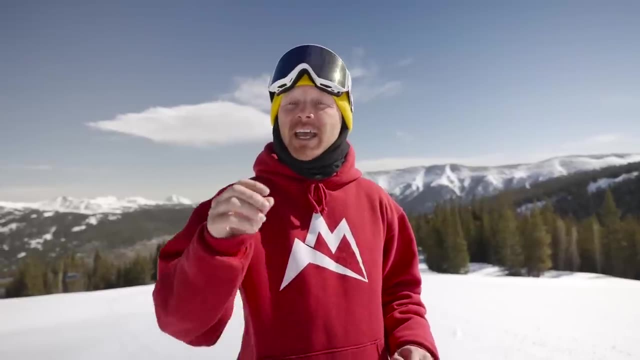 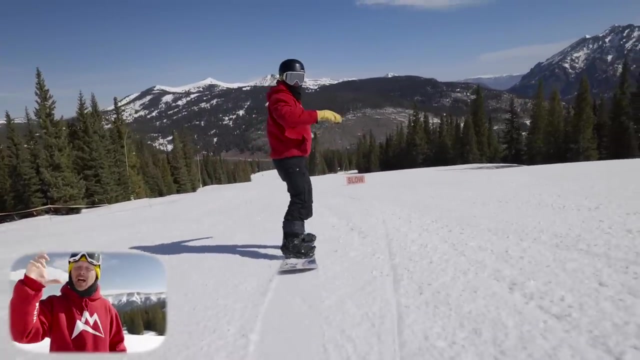 down. now let's continue on with this drill, but we're gonna once again make it challenging. we're gonna go back to a five count flat base. we're gonna see, within that five count can we do a full squat. meaning I'm really tall to start with and I'm gonna get as low as possible and stand back up while 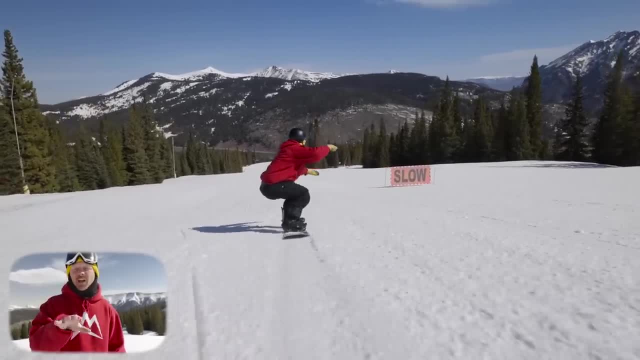 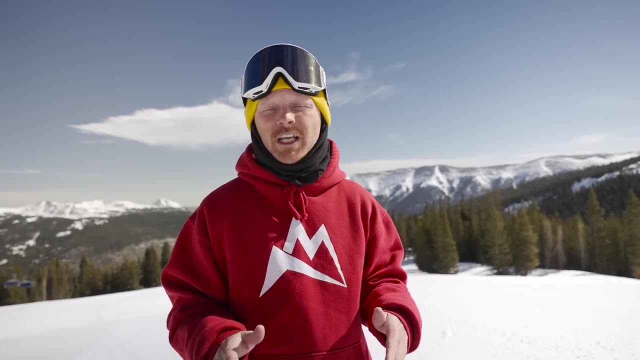 remaining in the strong stance while staying on flat base and not going edge to edge. but can I get low and come back up now? you may experience that you get on your toes a little bit too much. a lot of that comes from dropping your shoulders over your toes instead of letting your belly button sink down and 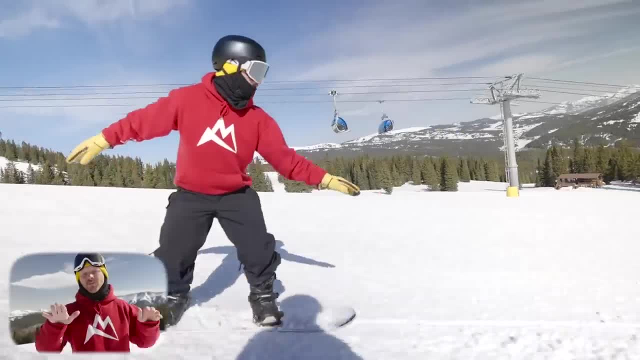 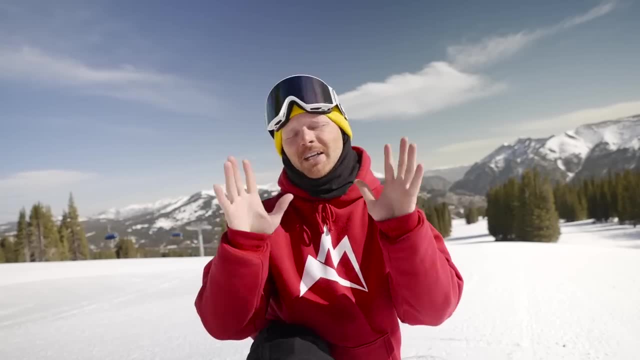 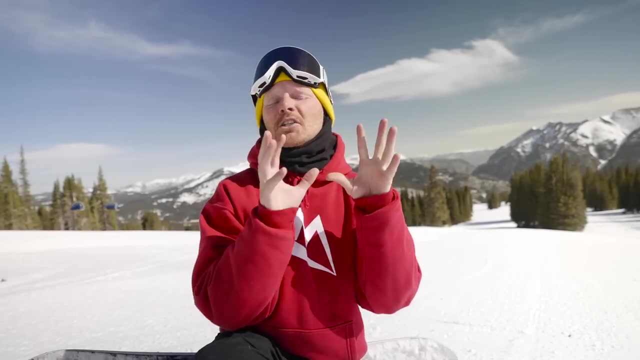 the goal is to sink your belly button down in a perfect neutral stance again, not too much weight on your toes, your heels, and get as low as possible. let's dive into a new drill. at this point you should feel pretty awesome about your stance and being flat base and use that as a drill, but not a common riding. 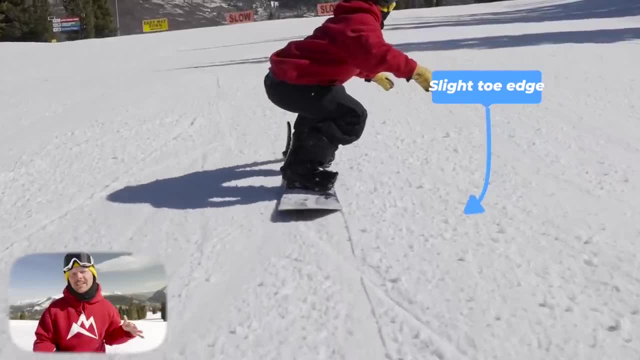 practice. so, with that said, instead of being flat base all the time, I actually like to be on a slight edge. whether that's toe side or heel side, I like to be on a slight edge. the reason why that is is because I am used to sitting on my feet all the time and I like to be on a slight edge. whether that's toe side or heel side, I like to be on a slight edge. the reason why 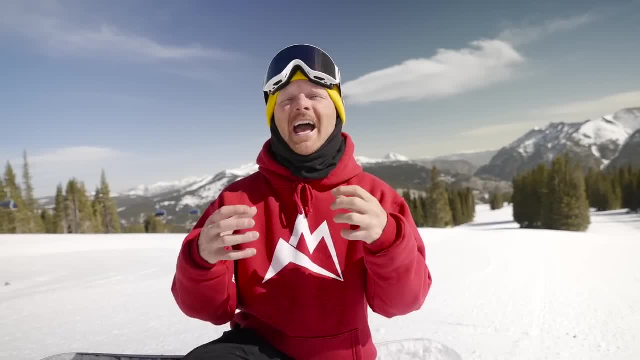 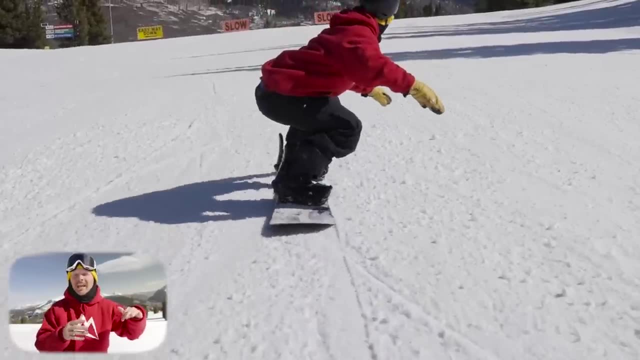 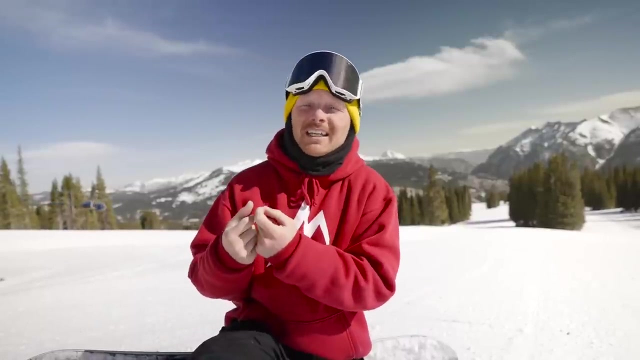 is if I'm on a slight edge or a slight carve. I have constant connection with the ground. more importantly, I have grip. now that grip allows me to turn quick, to handle terrain, to do a lot of amazing things at any given moment. now, sometimes our snowboarding is very reactionary and sometimes it's very you anticipate. 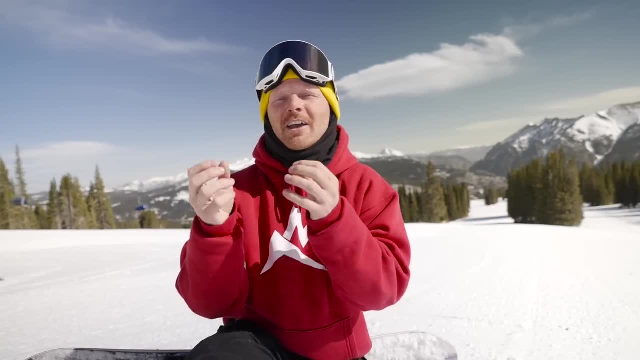 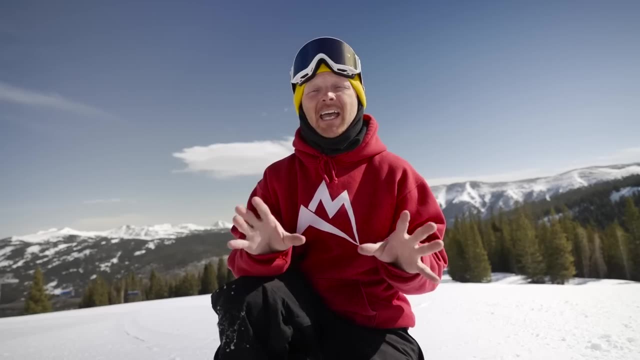 what's happening. but if I'm on a, on a slight edge, I can have the balance of both. now let's dive into some very similar drills, but with the emphasis of staying on an edge and creating grip as much as we can. so this whole entire time. 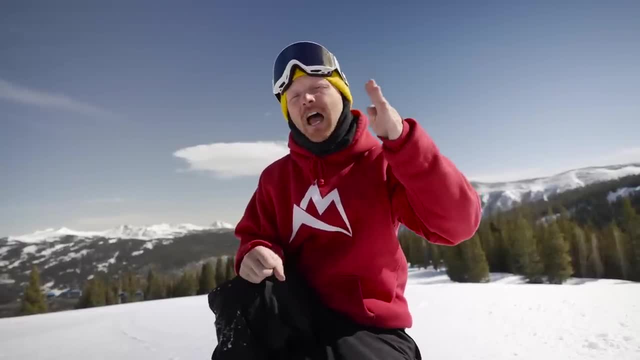 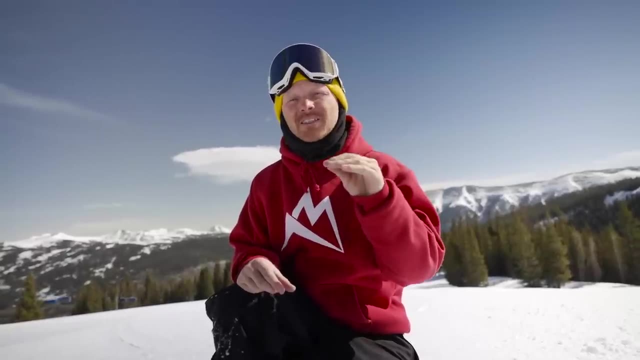 I'm not expecting you to have a gnarly edge. I actually want you to be in the opposite, where you have a very gentle edge, where you're still carving but it's not flat base. so I like to hang out around the five to even ten degree range. 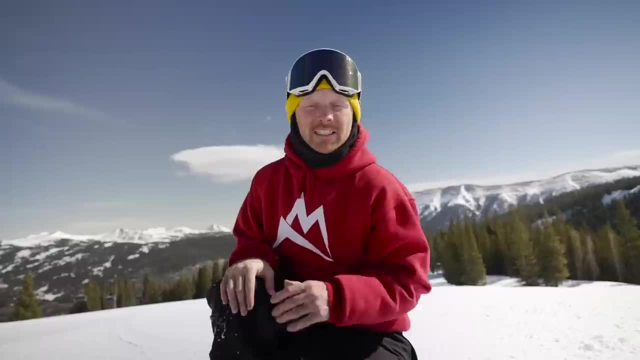 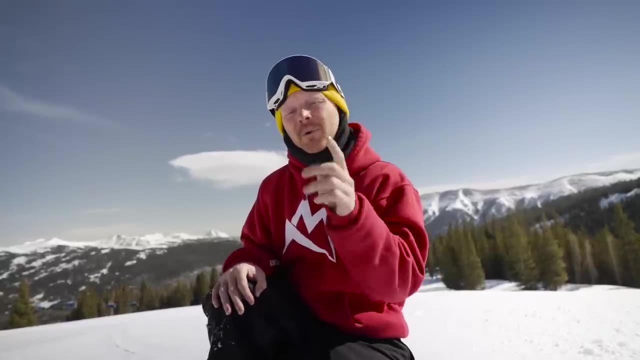 of tilt on my board for this next set of drills. once again, we're gonna be pointing our board down the fall line and we're gonna try to stay in a nice stacked position while being on an edge, but with the edge of the snowboarding. we're going to try to stay in a nice stacked position while being on an edge, but with the 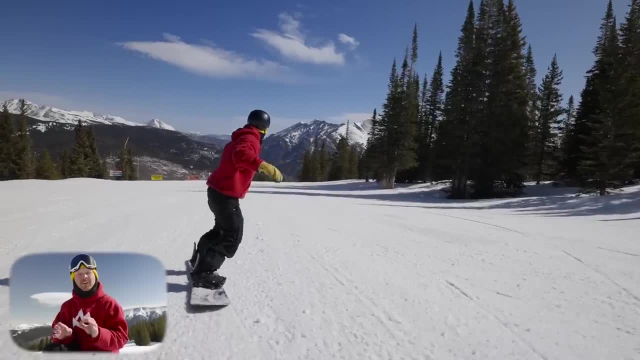 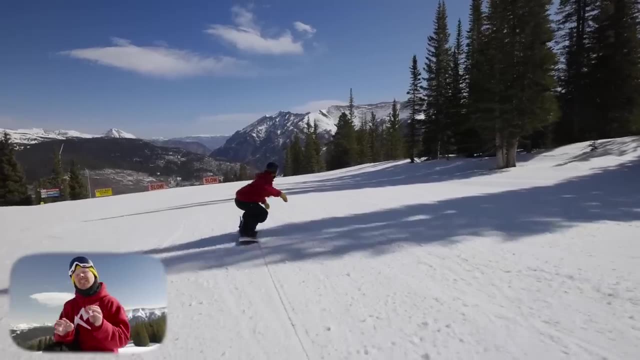 challenge and emphasis of try to create a straight, perfect line. now, this is really challenging because we do have a radial side cut. our board is designed to turn every time we put pressure on it, but this is more of a finesse movement, more than a power of movement. so the goal is to do a three count, one, one. 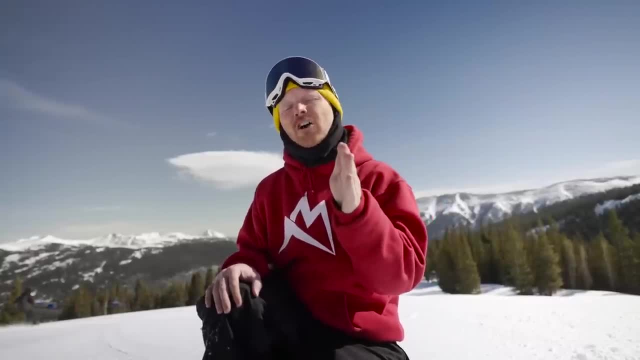 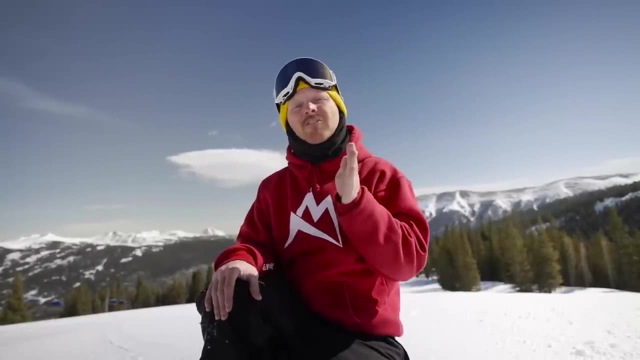 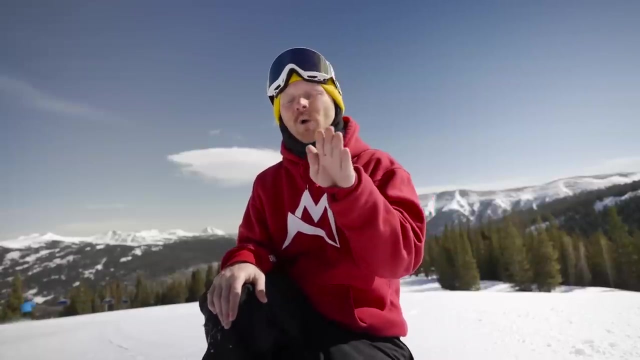 thousand, two, one thousand, three, one thousand. as you point your board down the fall line and then take a nice turn and look back uphill, what you should see is a nice gentle carved line. again. we're not seeing a flat base, wide path or trail in the snow. it should be a nice carve without making a 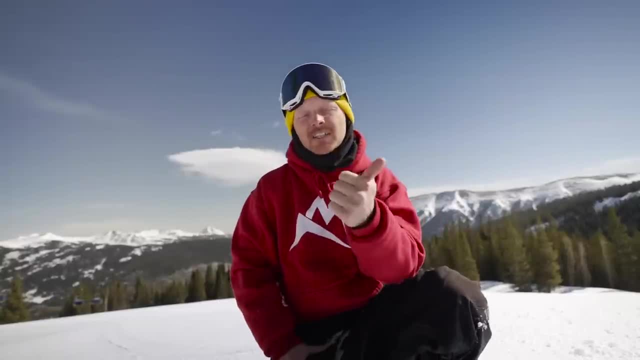 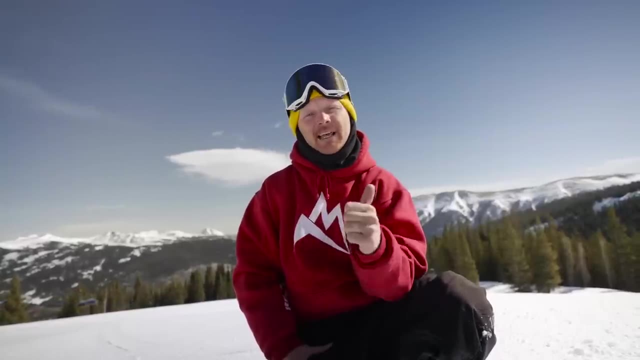 super abrupt turn. I'd love for you to do this for both your heel side and your toe side turn. once you're feeling pretty comfortable with a three count, then you're gonna go to a five count and then a seven count. obviously, as you transition into the five and the seven count, you're gonna start going really. 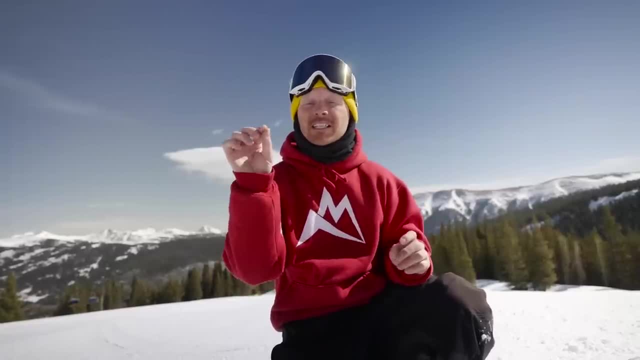 fast. but if you're in that strong body position and you're on a slight edge, you're gonna feel like you have extra grip and as I get faster and faster, I do like taking my centerboard and I'm gonna feel like I have extra grip and as I get faster and faster I do like taking my 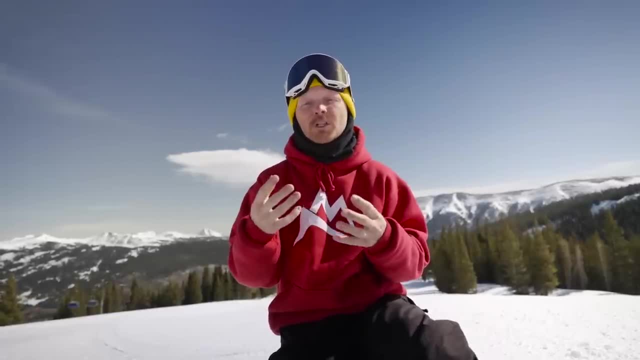 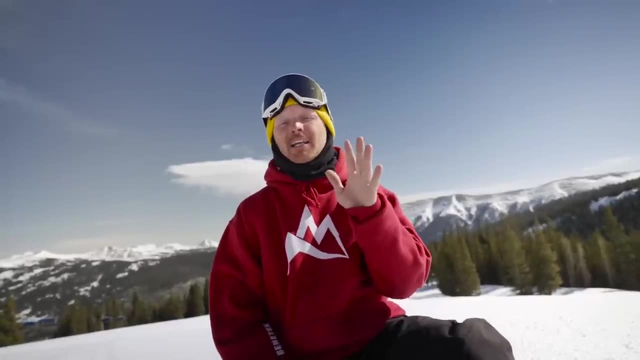 center of mass and getting lower, just so I feel like I have more range of motion. so if anything does come up that I can handle it like a shock in a car. now let's step it up just a little bit, not necessarily by adding more speed, but 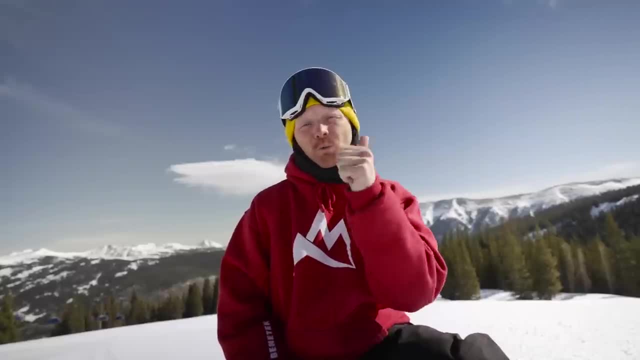 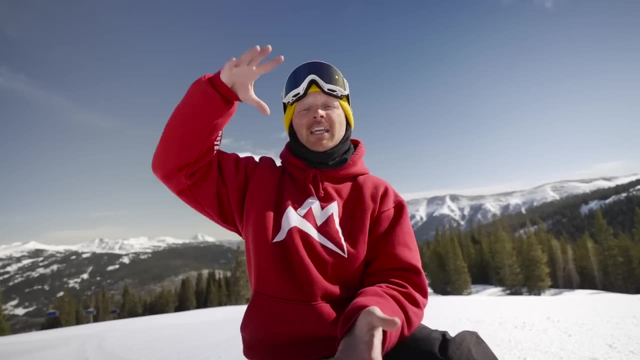 let's add more range of motion in your snowboarding. so we're gonna start with one squat, then three squats and then five squats, both on your heel side and toe side. what this is going to do is allow you to get in a greater range of. 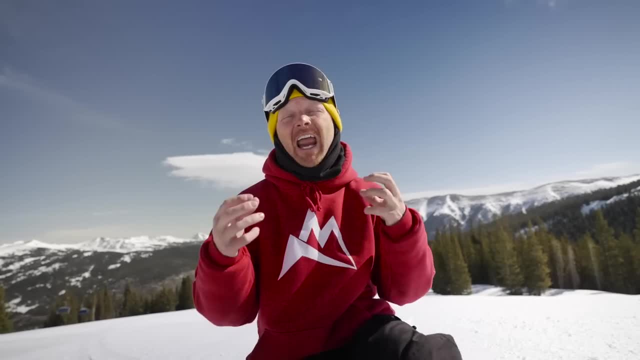 motion. so as you start going faster and faster, you can start handling a lot more terrain and a lot more power for your foot and your toe. so as you start going faster and faster, you can start handling a lot more terrain and a a lot more high speed maneuvers in a controlled environment. 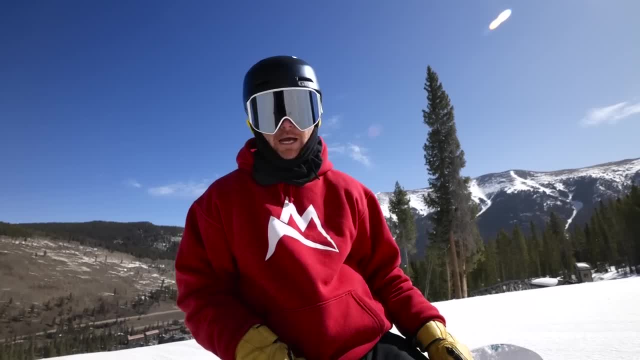 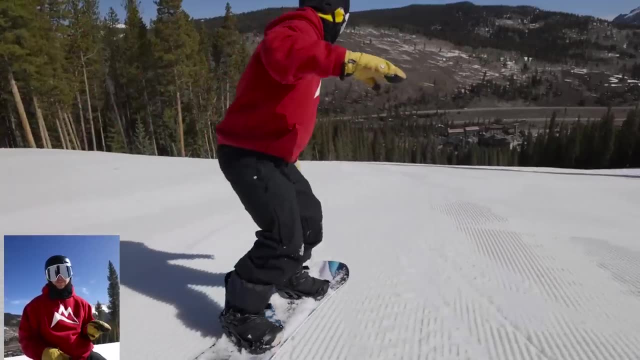 Now we've done a lot of flat base stuff and very one directional stuff, So the next drill we're gonna get into is making as many quick edge changes as possible while going straight down the fall line from edge to edge in a carve. This is extremely useful for when you need. 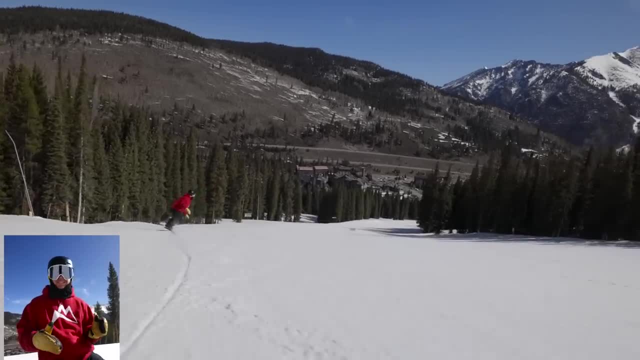 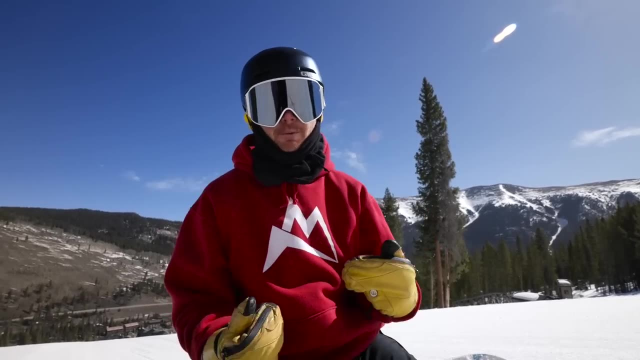 that panic moment to go from edge to edge. So let's practice it before we need it. But the number one key to this drill is your body position. I'm such a big advocate for strong body positions, so stay true to it If you are struggling with this drill. 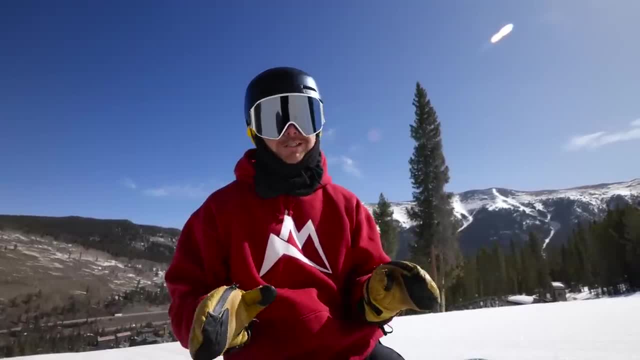 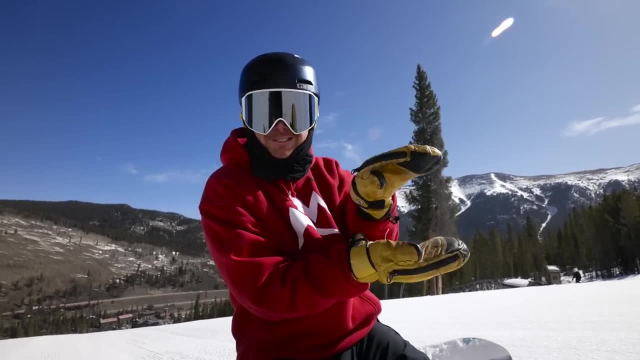 it's because you're not in a strong body position. You're making things worse. So the ideal body position is back to that original stance. get your belly button low and then you're gonna make rapid turns: heel to toe to toe, heel to toe and toe to heel. 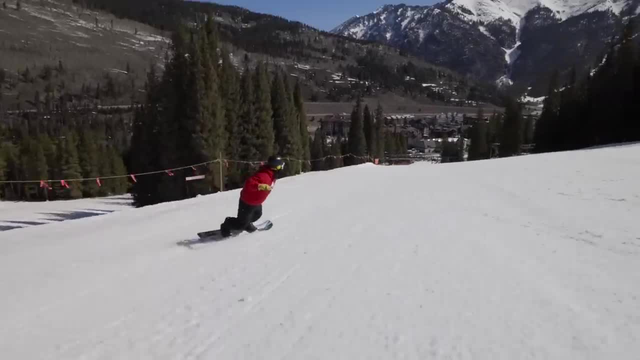 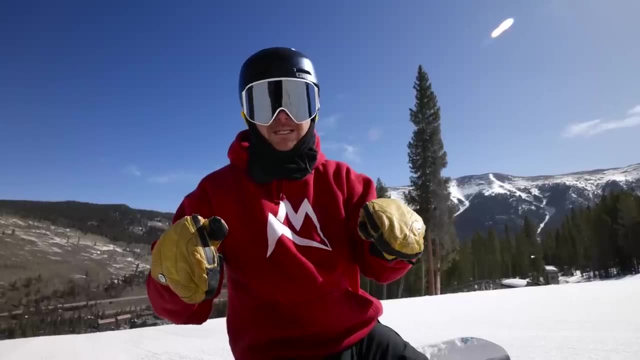 Now we do that by pressing our knees over our toes to get on our toe side edge. So to do the toe side edge, we're gonna press both of our knees over our toes, allowing us to engage that edge, and then we're gonna immediately push our knees back. 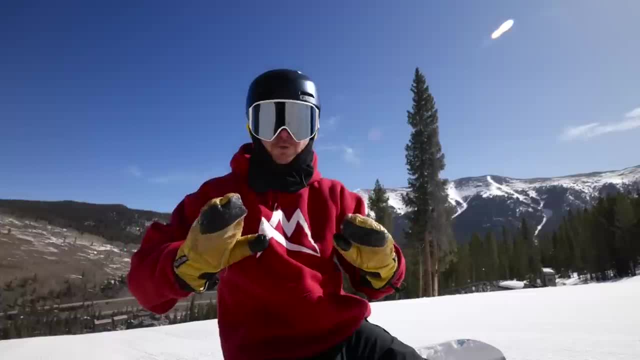 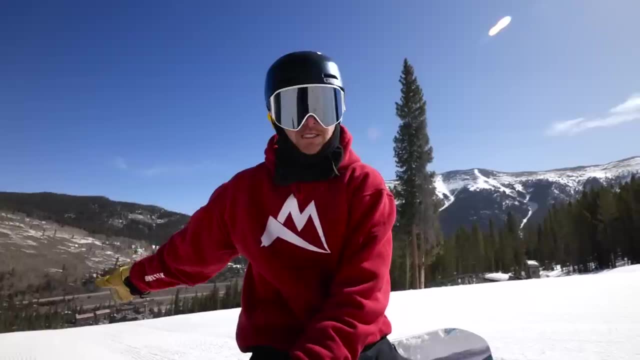 and lift up our toes and then we're gonna repeat that cycle back and forth as much as possible. Well, right now where I'm at, it's freaking slushy and amazing, so you're gonna be able to see the track and how easy and quick it is. 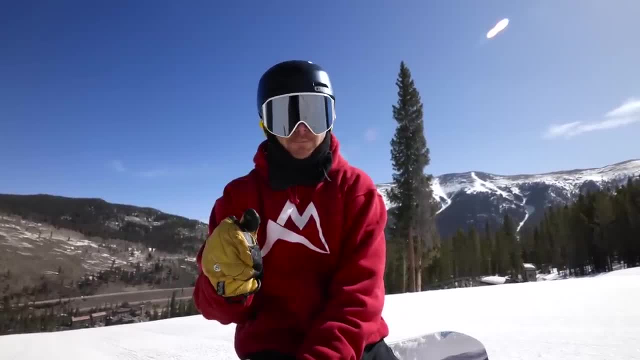 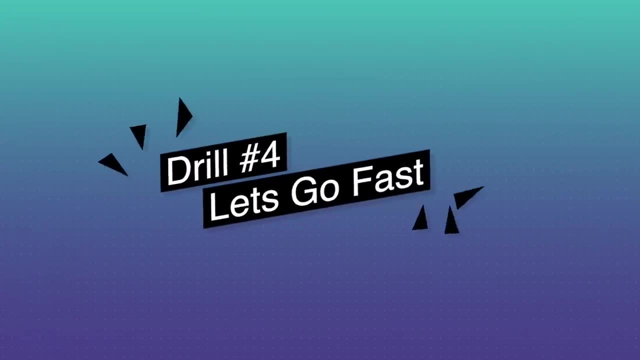 But this is extremely useful drill for those situations that you're not sure that you're gonna get into until you're already in them. So let's go. So our final drill is to actually go as fast as we can in a safe environment, At your own discretion. 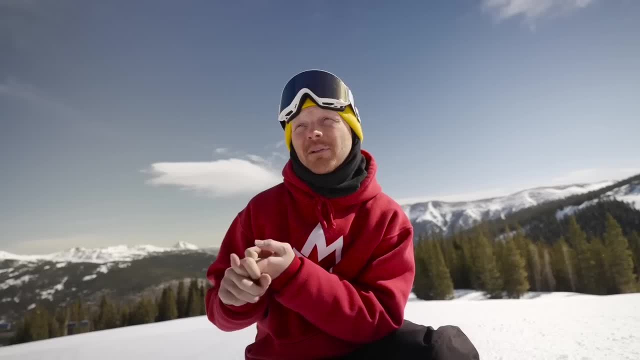 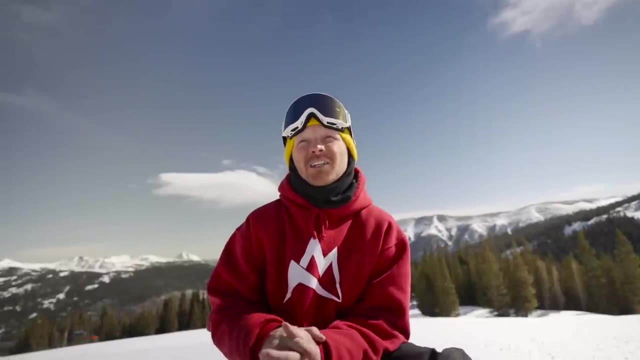 I'm not encouraging you to go fast and cut off ski patrol. cut people off like snaking people. Do this at your own discretion. So, first and foremost, you take responsibility for your snowboarding. But, as you're comfortable, try to go fast. 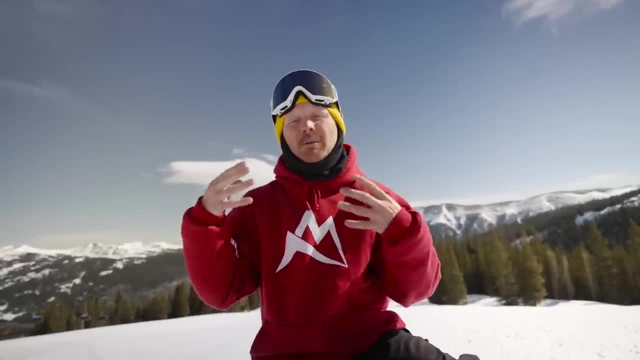 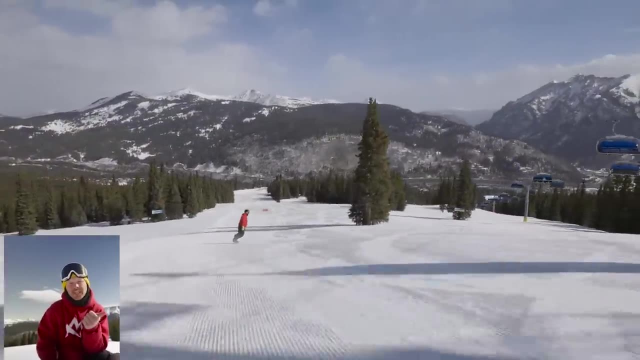 point your board down the fall line with a slight edge and I actually want you to get your belly button as low as you can and get into a nice aerodynamic position and hold that aerodynamic position for a three count, a five count and then a seven count. 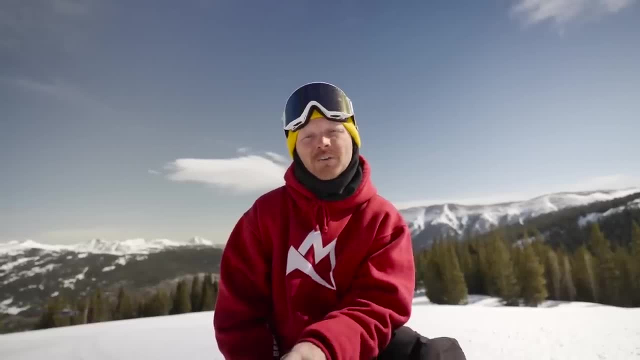 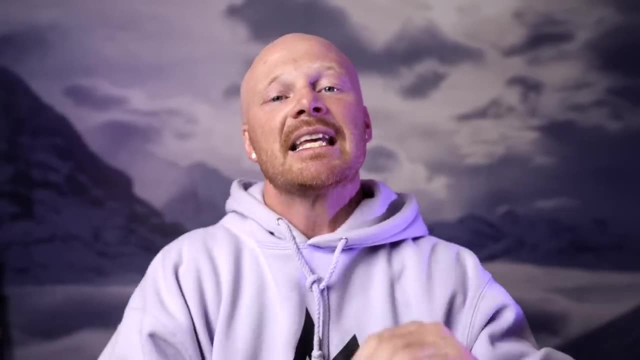 and then, equally as important, make sure you come to a stop and you're in control. Wanna maximize your season while preventing injury? If so, check out the link in the description below, where I offer two mobility classes and coaches classes every single week.